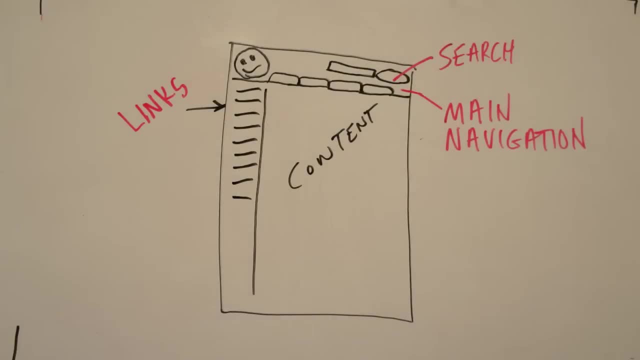 menu underneath. Most websites now also have search, which contains a search box near the top of the page with a search button immediately to the right of the box. These are all ways to make each website more accessible, while keeping the concepts simple and useful. 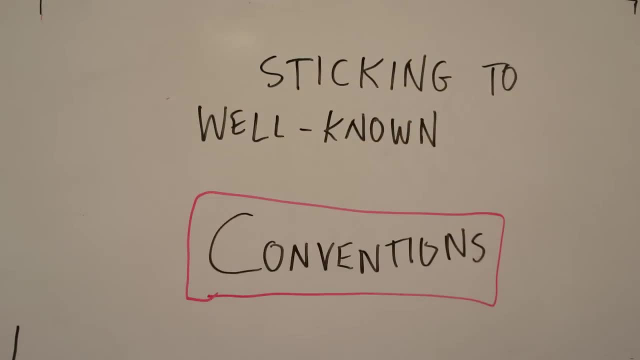 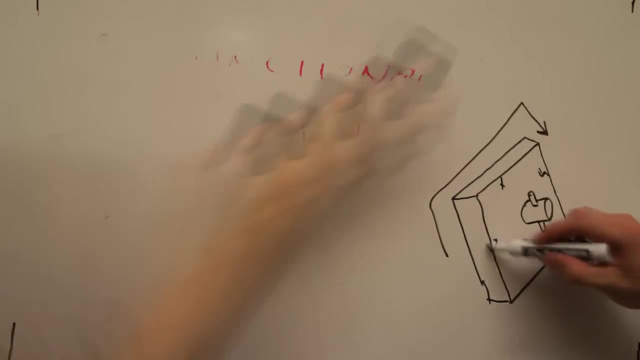 And sticking to some well-known conventions. The TEDS Value-Added model connects deeply with the core concepts of HCI, As described before. accessibility of technology is important, but as are many other traits that we must consider when we design a product. The model shows us the characteristics of why a certain person would choose one product over another. 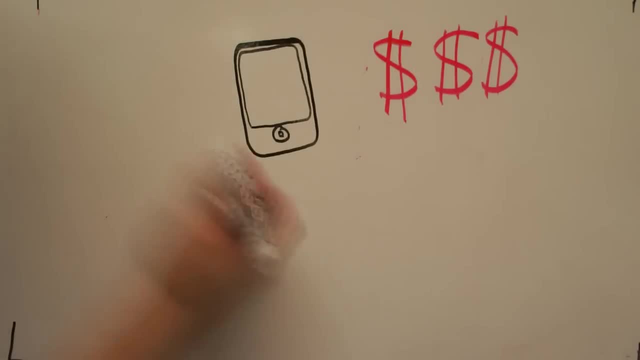 For example, ignoring cost. if the iPod has a more intuitive interface than some other mp3 player, more users will choose the iPod over the other mp3 player because it is simpler to use and makes the information that they want more accessible. Going off the value-added model, we can see the importance of value-sensitive design or VSD. 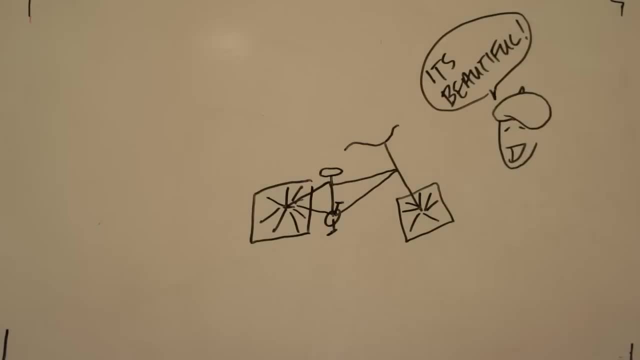 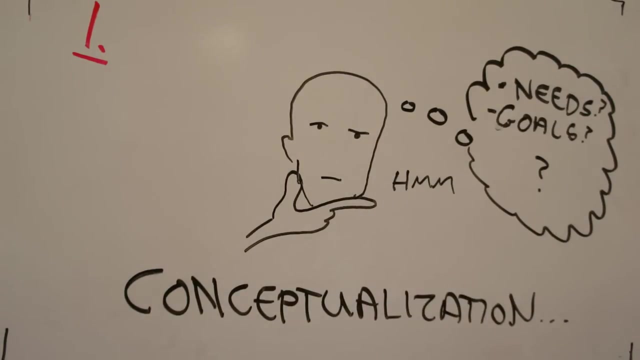 Where the end-users, not the designers themselves, dictate what they see as usable and intuitive. VSD is the approach to design of technology that accounts for human values. in the design process, There are three different traits. Conceptualization: which goals and needs do end-users have of our technology? 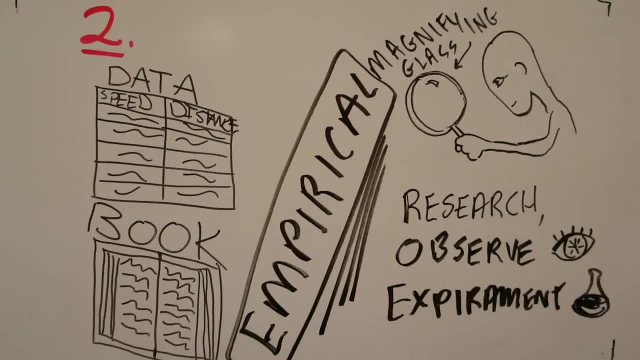 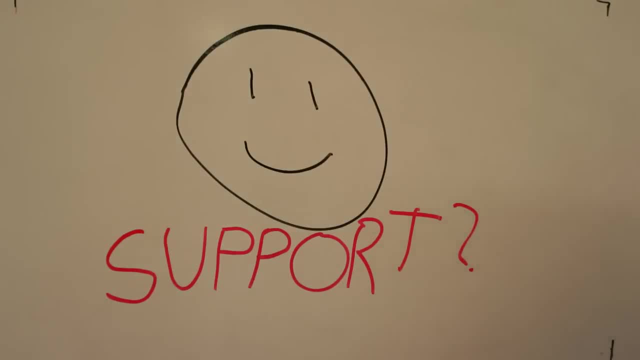 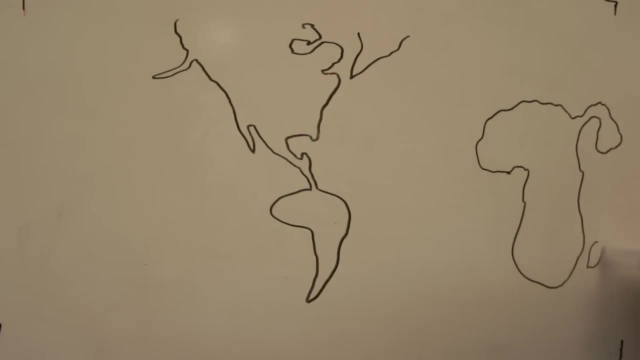 Empirical: what research and field studies have we done to prove that our design is preferable? And finally, technical: Does our technology support or hinder people's values? Implementing VSD allows designers to create technologies that adapt to different cultures and groups of people. 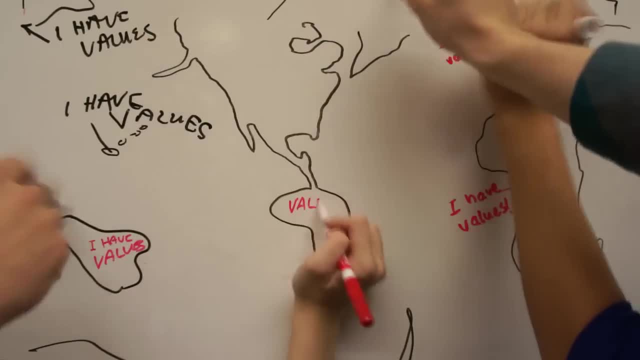 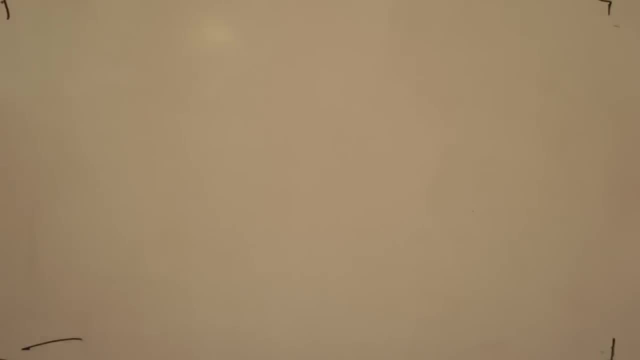 For example, one group may appreciate the convenience of having bank accounts linked to cell phones, where others may instead question the security of such a design. Human-computer interaction is the new wave of thinking and information To improve user experience. and how will we all interact with technology? 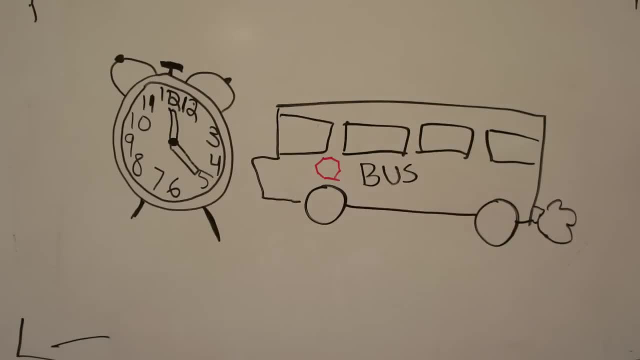 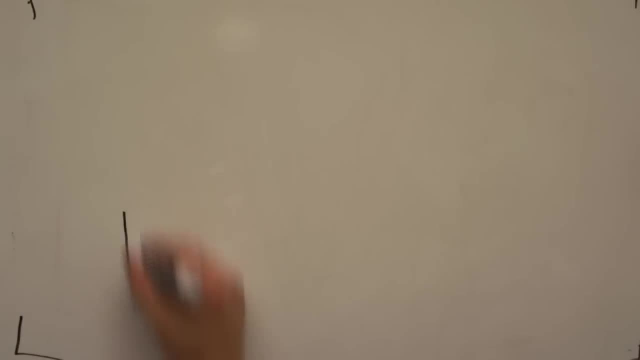 From the moment we wake up to the bus ride to school, to writing our late-night Info 200 papers, to relaxing in the middle of the day. The simpler and more accessible technology becomes, the easier it will be integrated into our everyday life.